specific distance from the earthquake in California. Other scales were developed in other situations to be consistent with Richter's. The Richter scale is logarithmic, meaning a magnitude 4 earthquake can be a magnitude 4 earthquake. A magnitude 4 earthquake is 10 times bigger than a magnitude 3.. Each whole number increased. corresponds with about 31 times more energy being released. The Richter scale isn't really used in the science community anymore. Its downfall, besides its specificity with how it can be used, is its inability to accurately measure large earthquakes. The Richter scale. is okay for measuring small and medium sized earthquakes, but it can't measure anything above a magnitude 8.. For this reason, the Richter scale is really only used by the media as a reference. The newest scale to enter the scene is the Moment Magnitude Introduced. 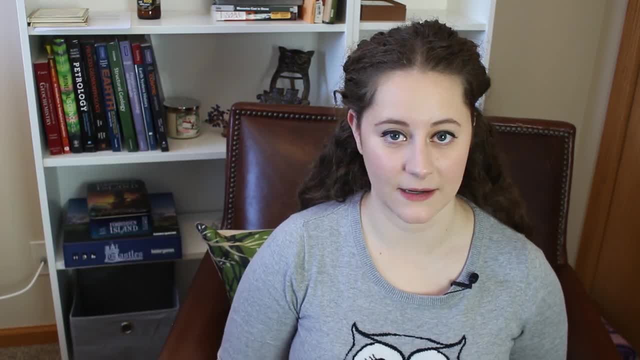 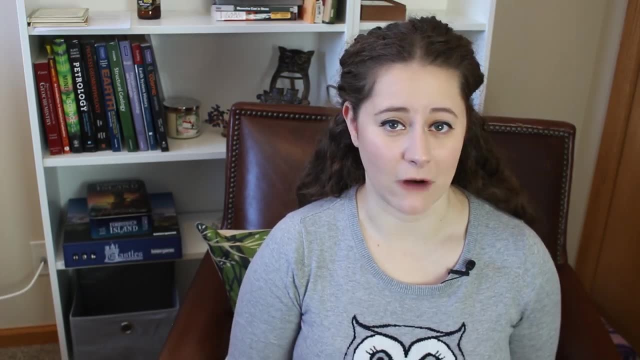 by Tom Hank and Hiro Kanamori in 1979.. Unlike the scales before it, the Moment Magnitude measures the size of a seismic event in terms of energy, specifically the amount of movement by rock. Because rock is a fairly consistent measuring tool, it can be used worldwide. 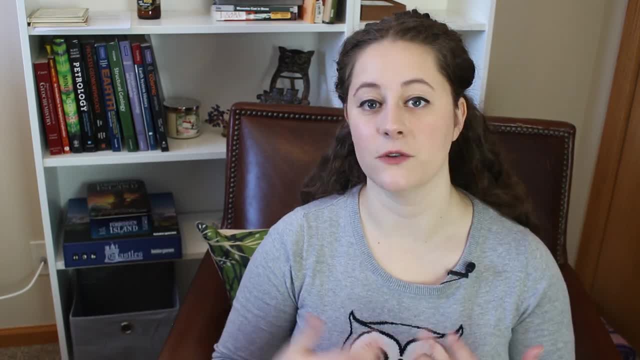 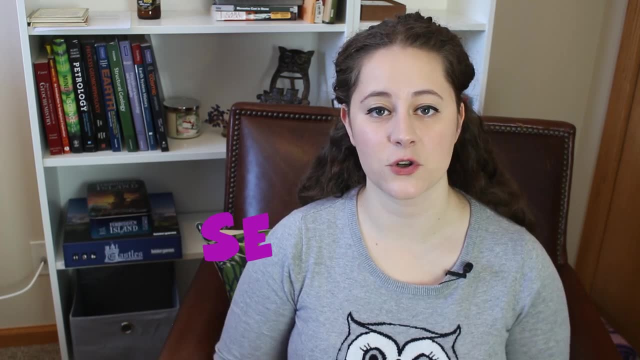 This scale is also logarithmic, so, like Richter's, a magnitude 4 earthquake will be 10 times bigger than a magnitude 3.. To reach the magnitude of an earthquake using this scale, you will measure the seismic moment, which is equal to the rigidity of the earth multiplied by 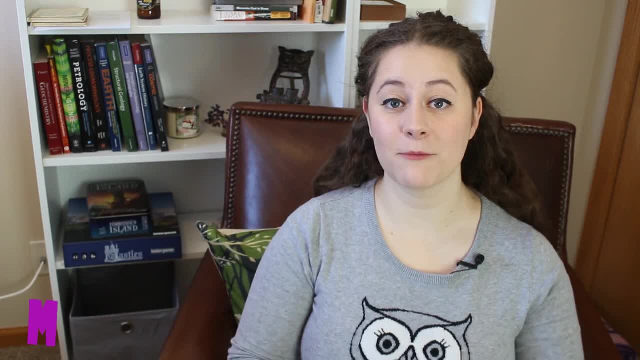 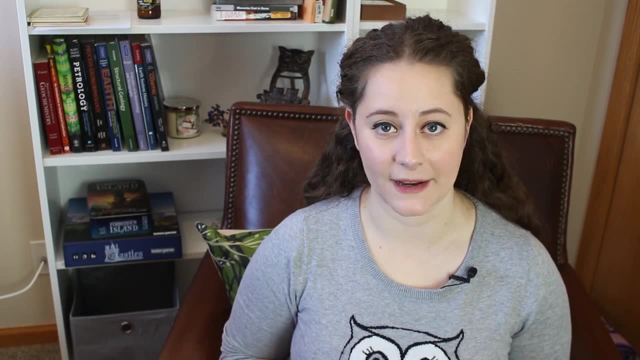 the average amount of slip on the fault and the size of the area that slipped, And you will then plug it into this equation. The Moment Magnitude is the most widely used scale by geologists today because of its consistency on a global setting. It can also measure large. 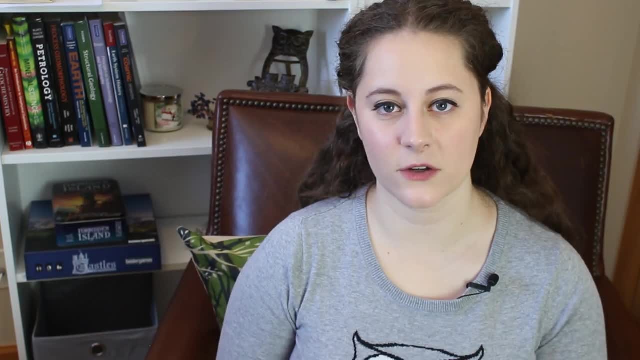 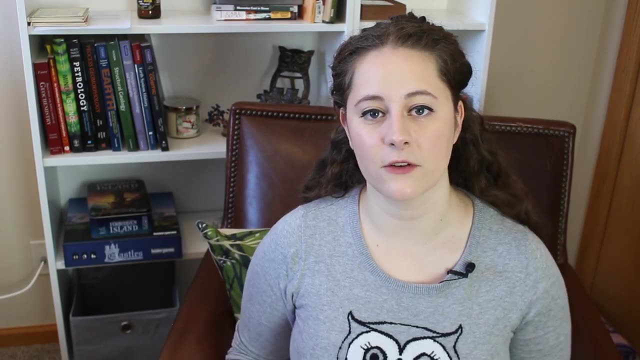 earthquakes much more accurately than Richter's scale. So while historically we still use the Richter scale, we use the Moment Magnitude to study modern earthquakes. We're slowly getting all we need to know about earthquakes. If you've missed another video in the playlist: 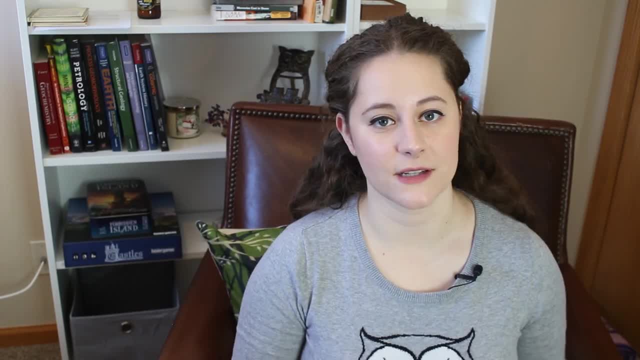 I will link it here. Next time we'll be talking about the effects of earthquakes with some examples. for good measure, Be sure, if you have specific questions about earthquakes, you can leave them in the comments below If you want to learn more about earthquakes. 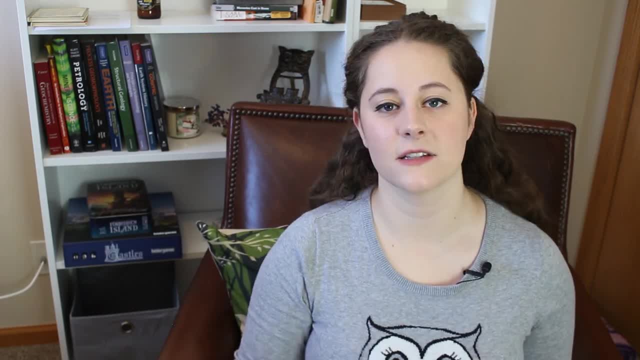 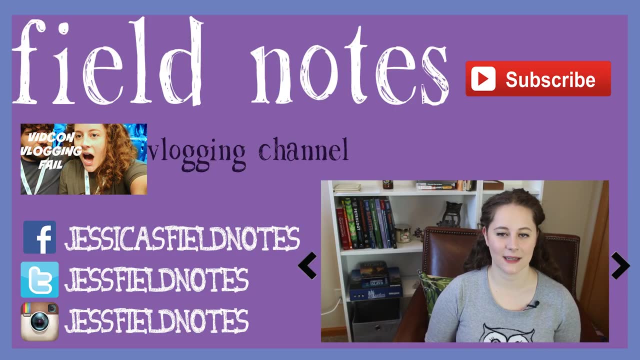 leave them in the comments below. Remember to like this video. if you liked it, subscribe if you would like to see more and I will see you next time. This was developed by Giuseppe Mercalli in the early 20th century. I said earliest. I was an Italian seismologist and didn't have the a-. oh god, I feel like. 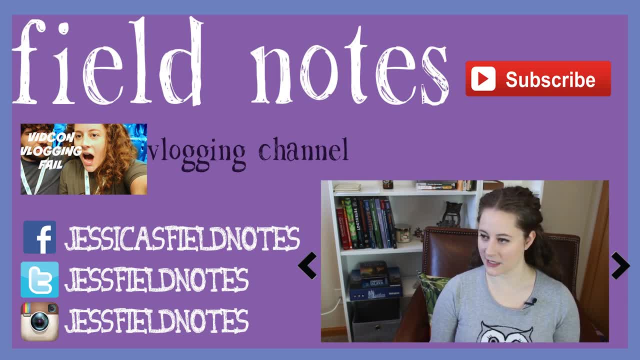 you tuned me out until I say: yeah, Is that okay? Does that make sense? Okay, This scale is not used very much anymore because of what You like. talk about something or you say something long enough and you're like: is that what it's called? 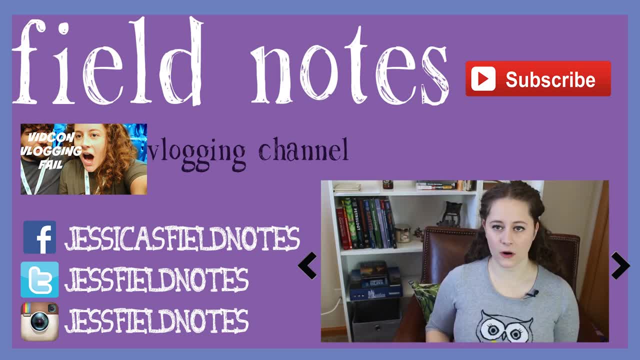 Is it a scale? What are you?